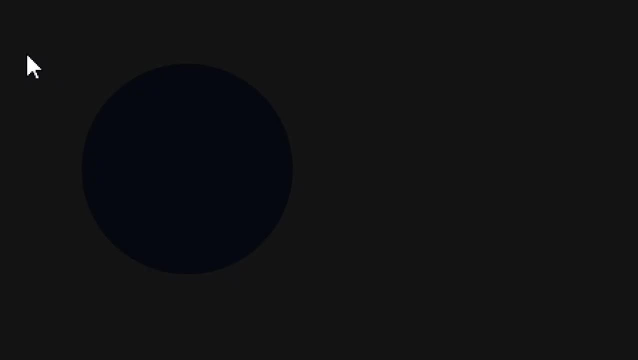 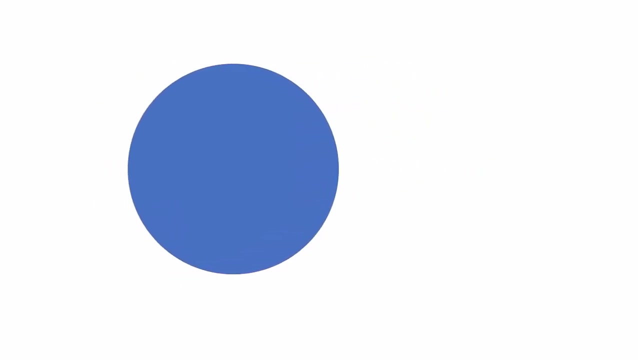 see what happens when we select the morph transition. Let's see what happens when we create the preview for this, So as you can see it smoothly transitioned from one position to another, Just make sure that you use the same element for both slides so that the transition. 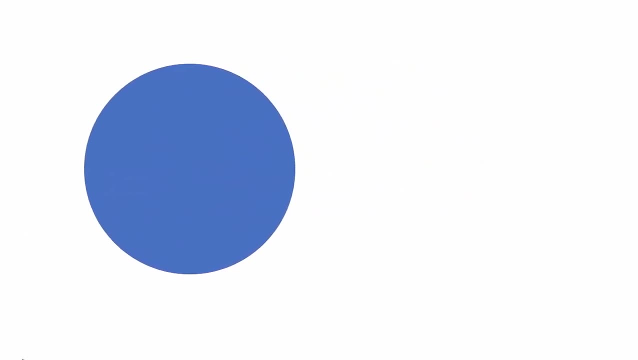 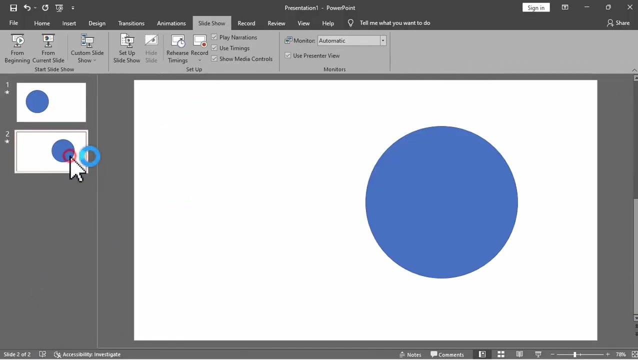 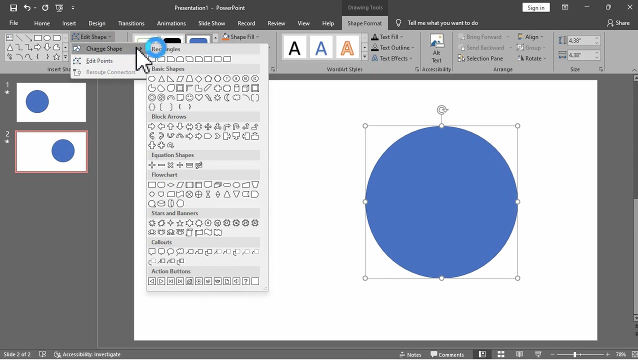 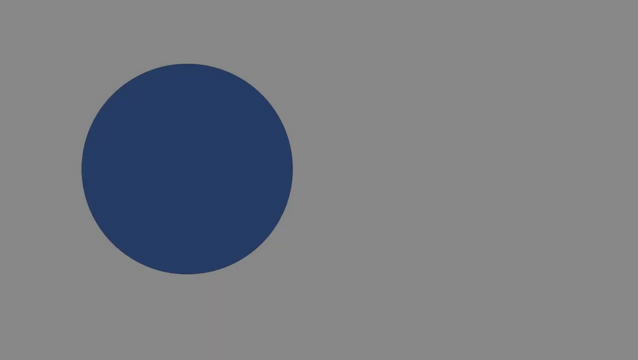 appears seamless. Now let's attempt to change the circle shape to a triangle shape and determine whether it works as intended. We can change the shape of the triangle shape to a triangle shape under the shape format tab, Since the two shapes are completely different from slide 1, which is a. 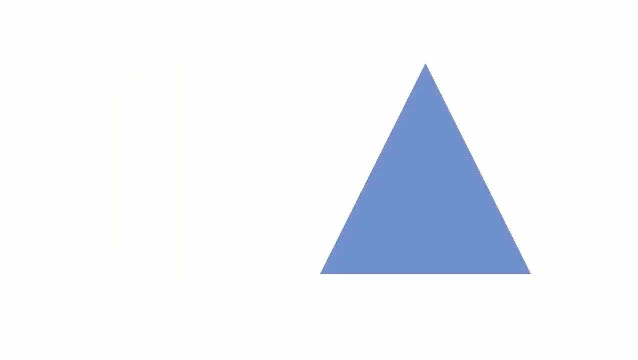 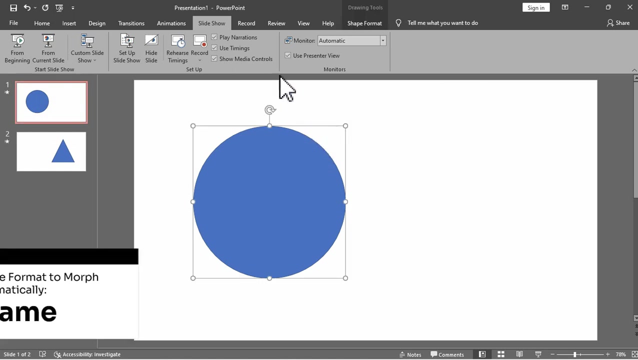 circle to slide 2, which is a triangle, the morph transition will not be visible. However, we can still perform a morph transition between these two different shapes by using the appropriate naming scheme. To accomplish this, start the object name with two exclamation points and assign the same. 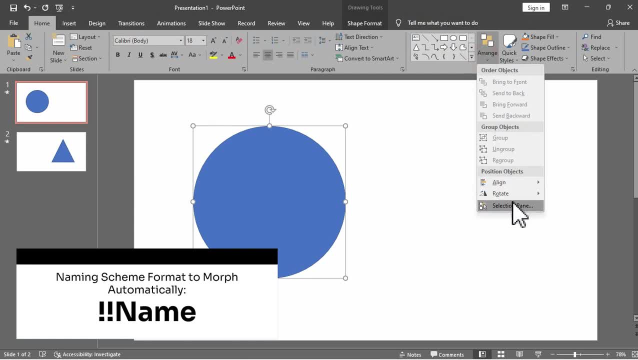 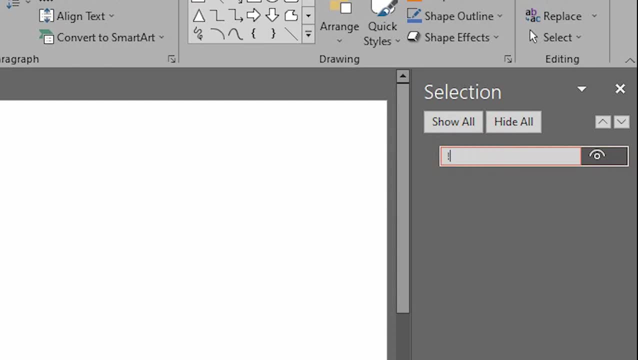 custom name to the two objects. So let's start the object name with two exclamation points and assign the same custom name to the two objects. You can alter the name of the shapes by navigating to the home tab, then the arrange and selection pane. For the transition to function properly: the same name. 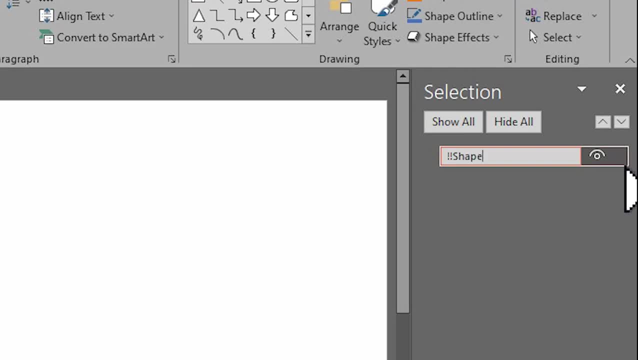 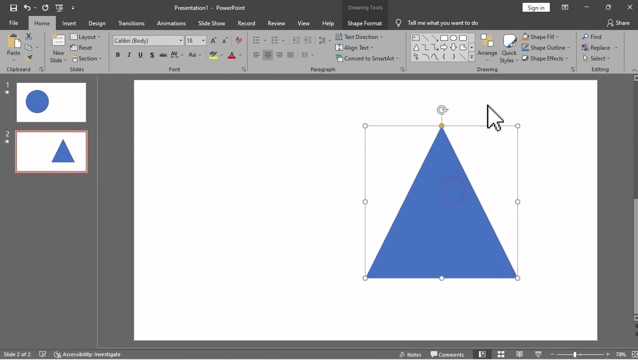 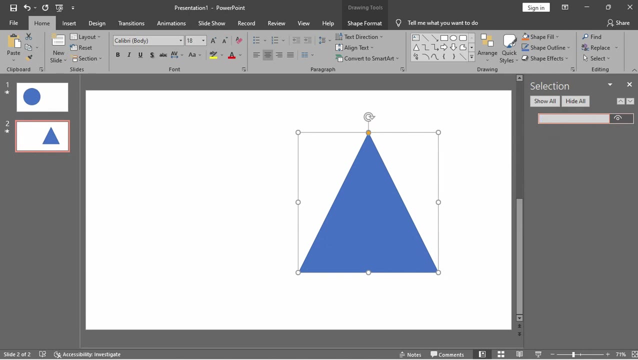 must be assigned to both objects in the selection pane. We will apply the double exclamation format. We will copy this name from the circle shape and then paste it on the second slide. for the triangle shape, We will just paste it here, which is basically the same name for the triangle shape. 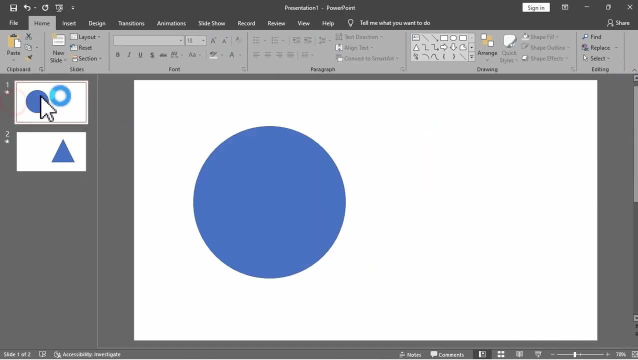 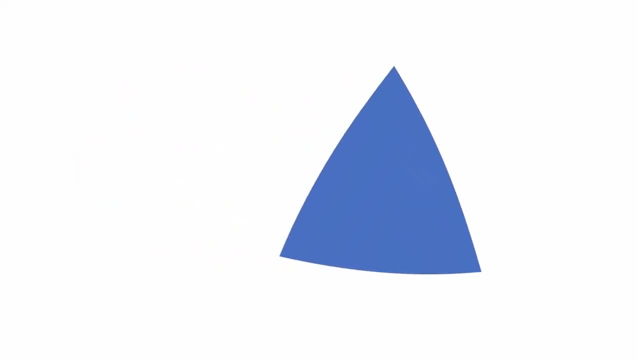 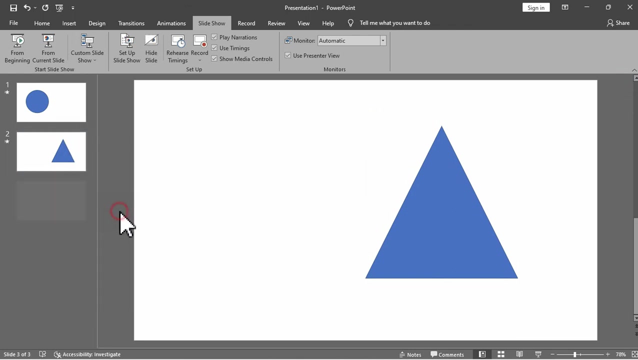 Now let's see if it worked this time and, as you can see, it is successful. We can view the morph transition between two different shapes, as long as they have the same naming scheme in the selection pane. Now, to enable the triangle to exit, we will duplicate the second slide To accomplish this. we will move. the triangle to the right or beyond the circle shape from the selected canvas. You can also talk with setting. the includes here two of terms. For example, if you want the boxes to my space with multiple interactionleton bars from the Duplex method, we will apply the equalization method In the shells, будеına is added image为 fundamentally. in your drawing, In the shells, where you Please make a translation, In other words, the Momo though is applied. Anふs Institute, support our skill, you who knows to use it. I have to do another example to start the explanation, but since I have to, 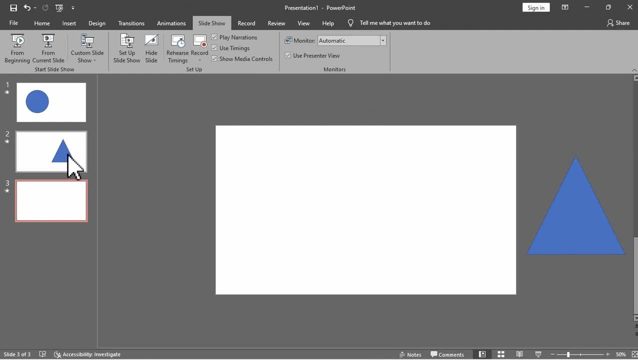 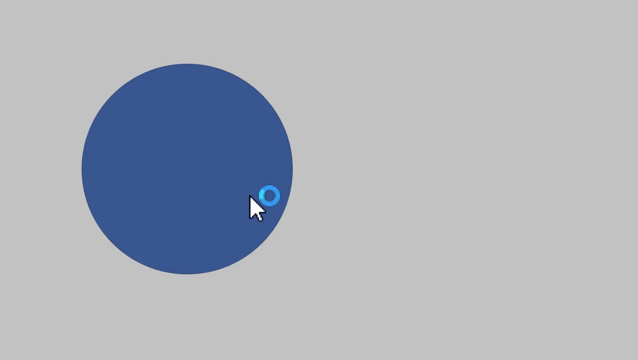 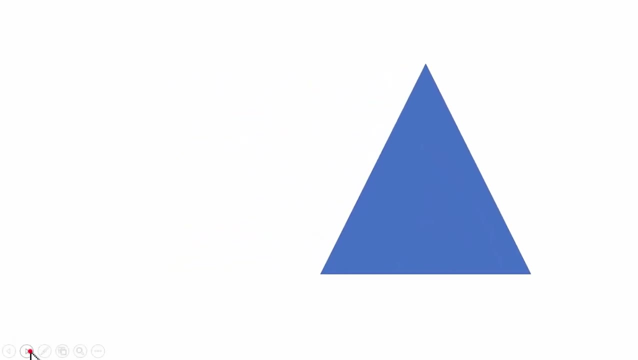 slide under the slide three. as you can see, the triangle in the slide two is in the right side of the slide and the triangle in the third slide is outside the slide. so here is the final outcome: from circle in the slide one to triangle in slide two and the triangle will exit in the slide three. 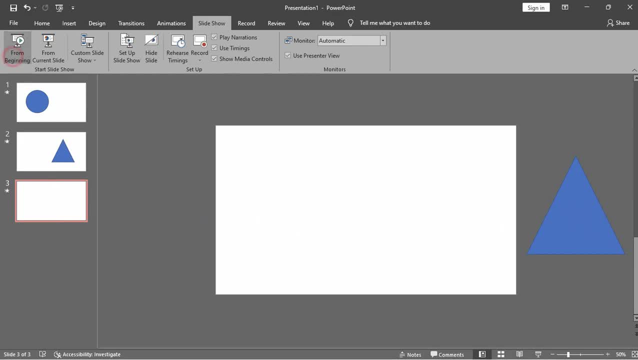 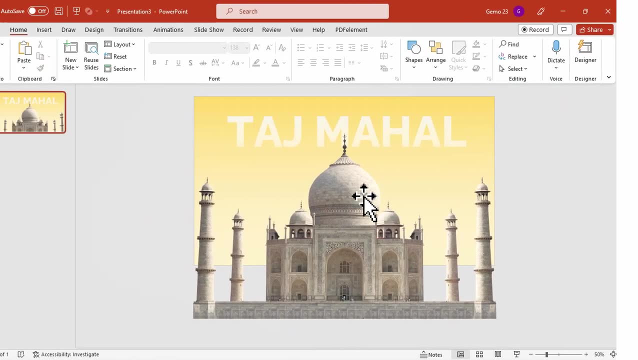 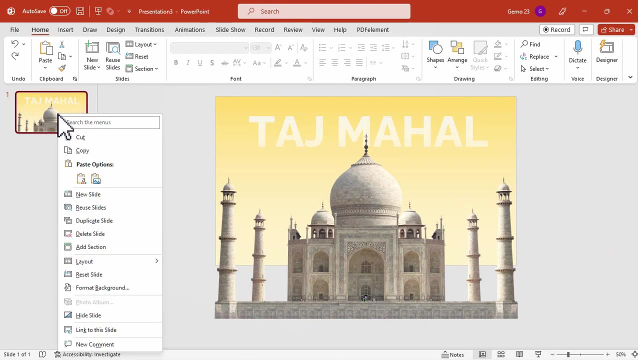 so that is how the morph transition actually works in microsoft powerpoint. now let's attempt to design an actual presentation with morph transition. i currently have a transparent picture of the touch mahal and a title text. to initiate the morph transition, we begin by duplicating the slide. we can now proceed to. 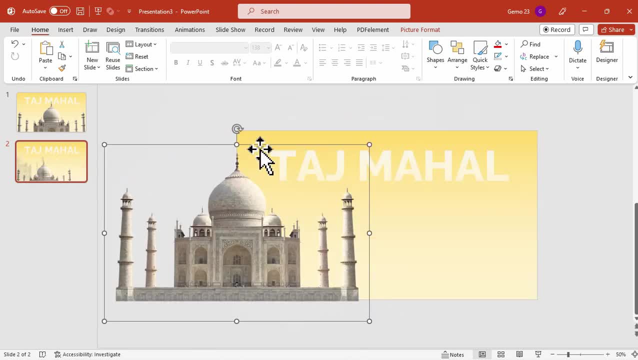 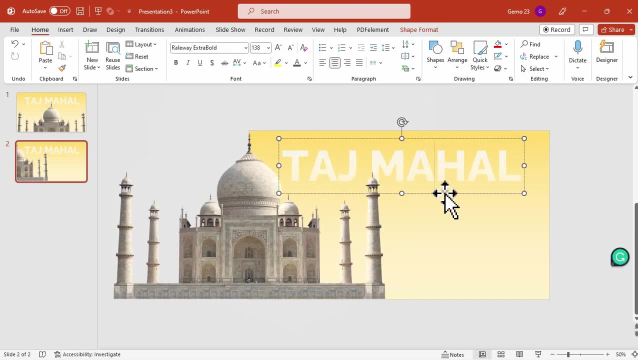 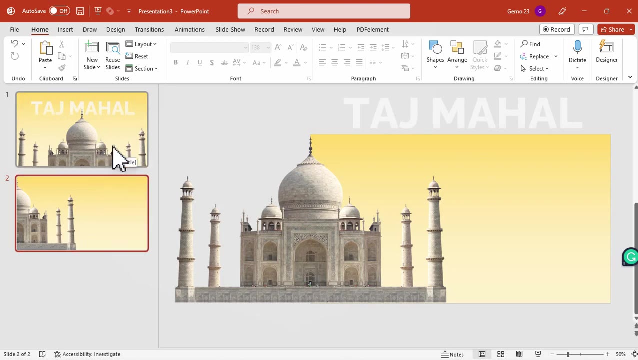 reposition and resize the elements in the second slides. as you can see, i move this touch mahal picture on the left part of the slide and we will move this title text outside the slide in the second slide. please observe the positioning of our photo in the first and second slides. 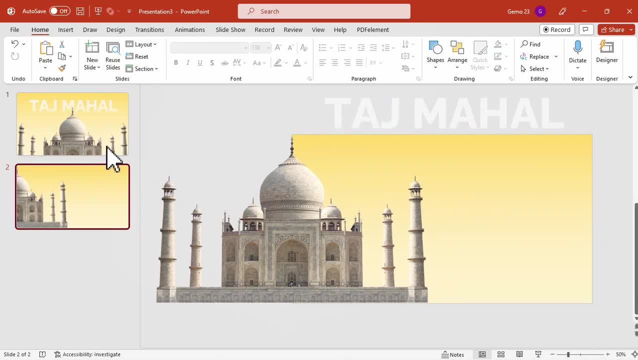 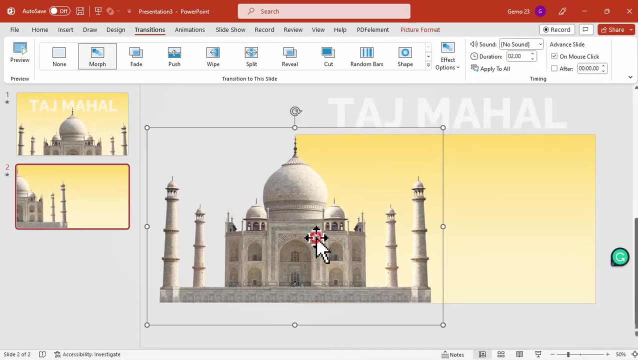 then we will apply the morph transition to all slides. as we apply the morph transition, these elements will blend together smoothly. the position of touch mahal moves from full scale in the first slide to half in the left part of the slide, since we resize and reposition it. the morph transition follows the same process. 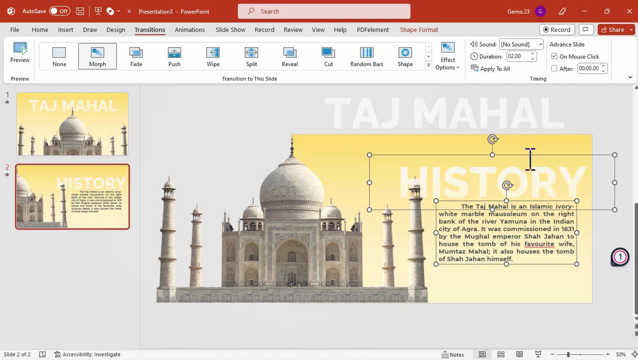 as keyframing in other editing tools. now i have added here another text to the second slide and i will send it to the back as a layer. as you observe, the morph transition for the newly added text is just a simple fade transition to make it more interesting, we will also apply the morph. 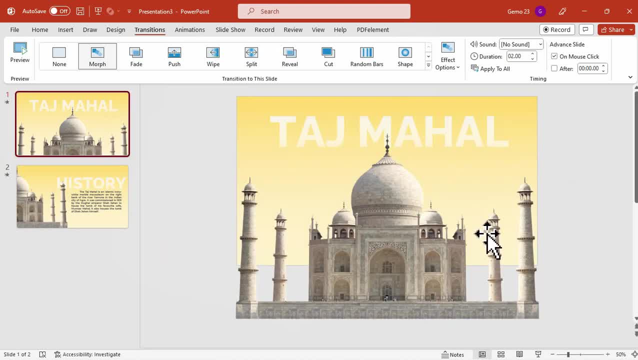 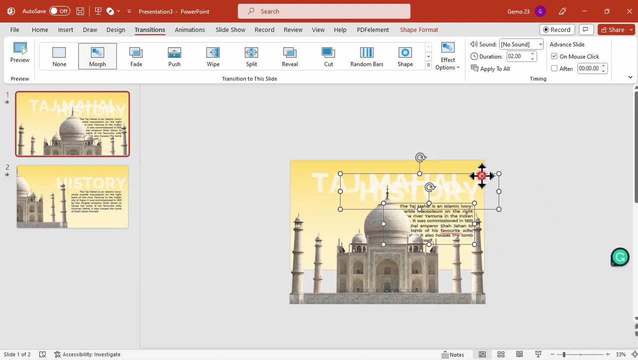 transition to this text. we will just copy this text and paste them on the previous slide, then send them to the back for layering. next is to move this text downwards, so that whenever we move this from the first slide to the next, the direction of this text will come from below. 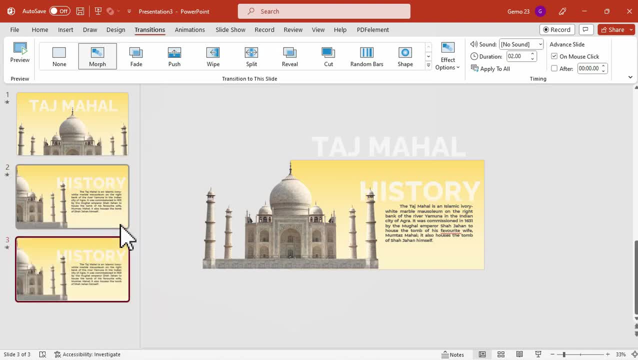 so let's proceed with the tutorial by duplicating the second slide and then adjust the placement of the elements to achieve a morph or blending effect. specifically, we will move the text, or the history part, upwards, so that its direction is just the transition from the second to the third slide. and then, as you can see, here's the 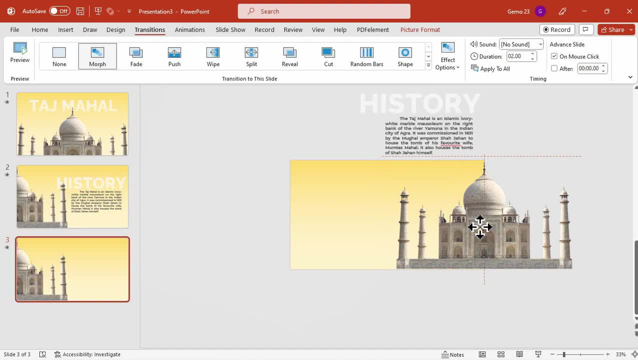 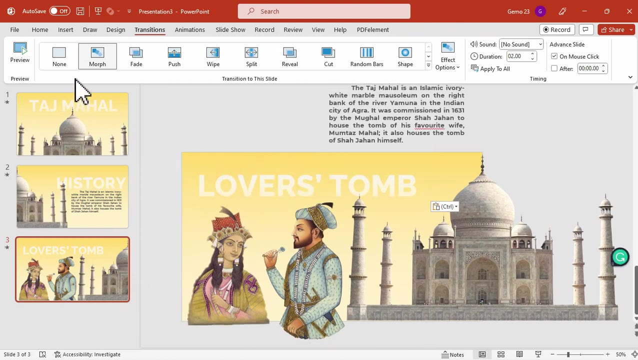 preview for that, and then we will move this picture from left part of the slide to the right, so that the movement will be from the left to the right. we will also add a picture, and these pictures are not yet included- in the second slide and, as you notice, the transition for these pictures are just like 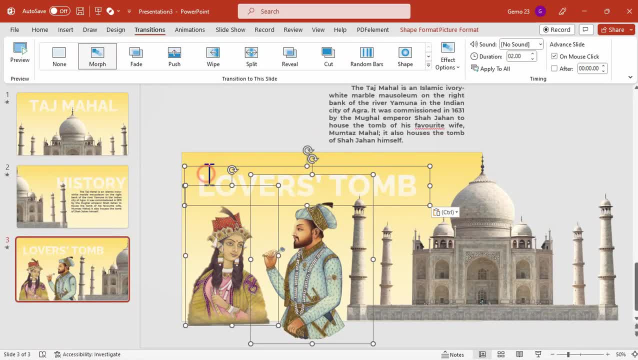 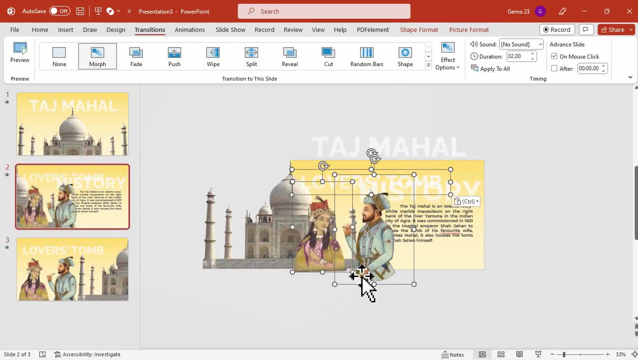 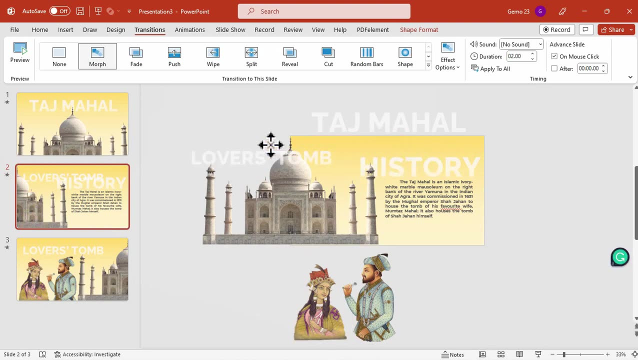 the fade transition. since these pictures were not included in the previous slides and to apply morph, we will copy that elements and paste it in the previous slide or in the second slide and then we will move this picture downwards so that the starting position for this will be from below if we shift from. 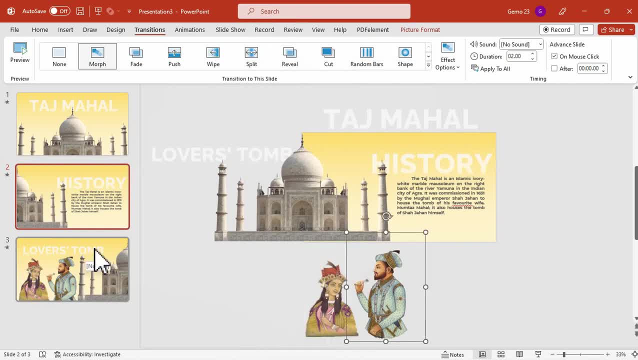 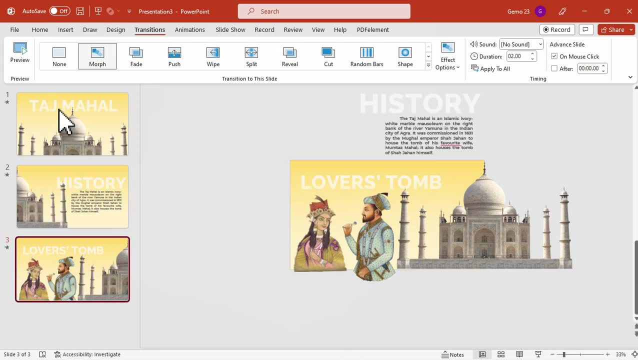 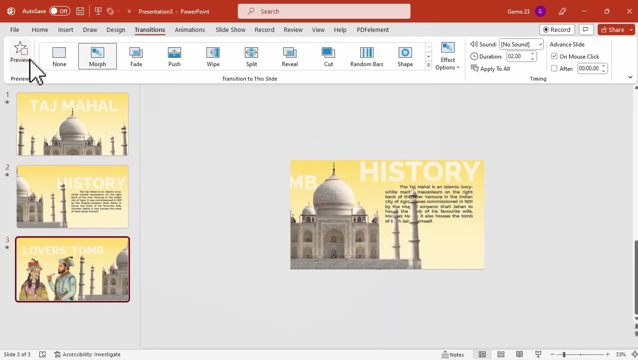 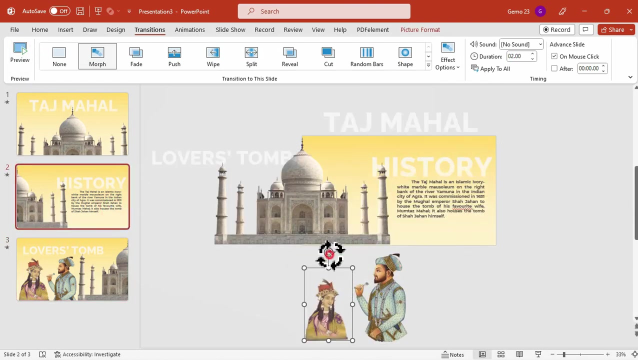 second slide to the third slide and then the text. we will move it in the left part and here is the preview. now let's try to adjust the layering for this touch model for more seamless results, and that's perfect. we can also resize these pictures or rotate it for more dynamic effect for the morph. 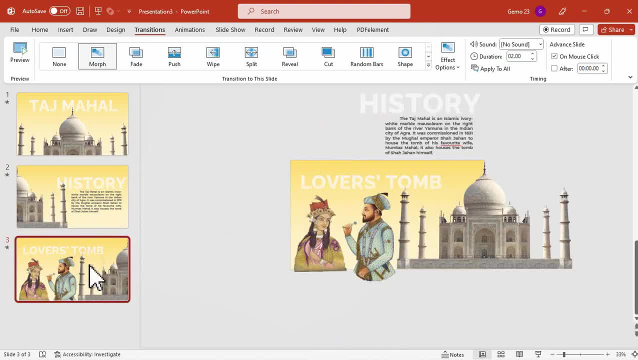 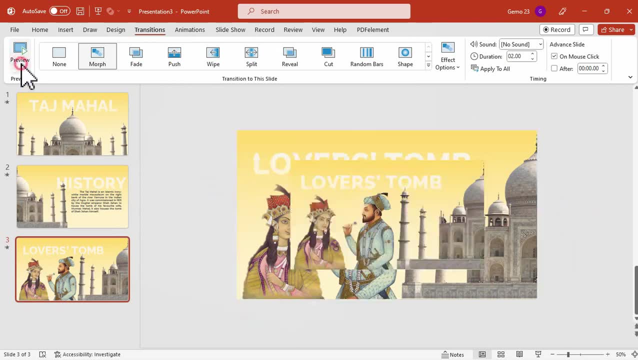 transition, and here's the preview. keep in mind that morph transition will help you make smooth animations, transitions and object movements across the slides in your presentation, in the second slide, in the next slide. you will also want to make some adjustments in the second slide in order to match the 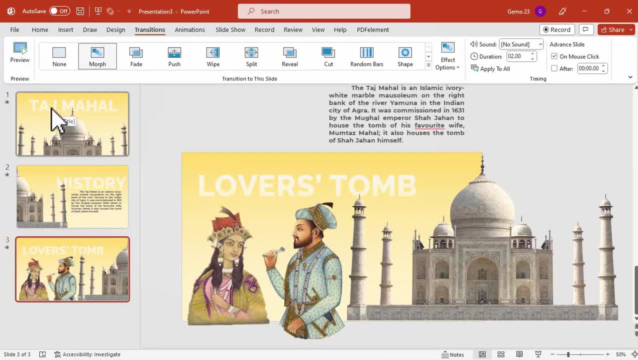 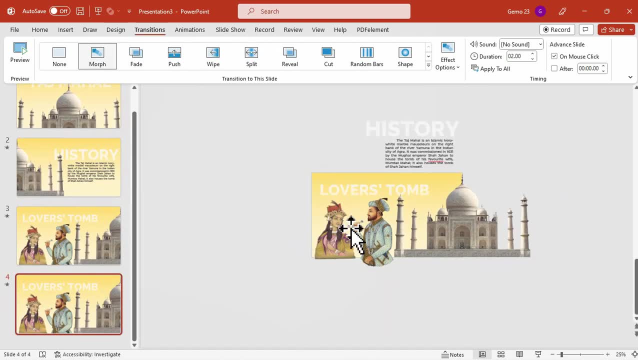 in your presentation. Now let's try to duplicate the third slide and reposition our elements once again. We can delete this text box, the history part, since these texts are not involved in the third slide- and this lover's tomb text. we can move this upwards and then, for the time for the 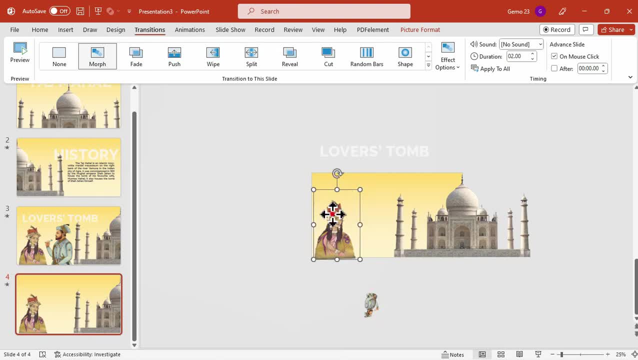 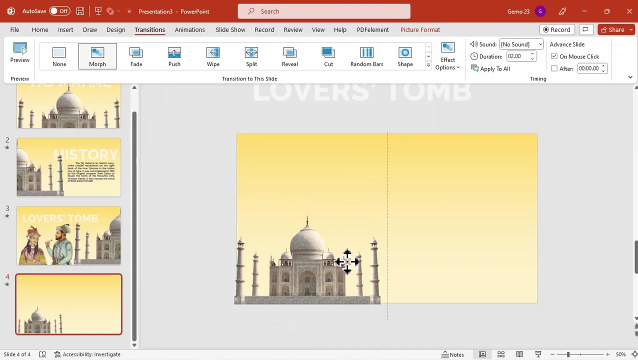 exit for this picture. we will rotate it and move it outside the slide And now we can see the preview or the exit for the lover's tomb text and for the pictures. And now let's try to reposition and resize this Taj Mahal PNG image once again, And we will move this in this part: resize the. 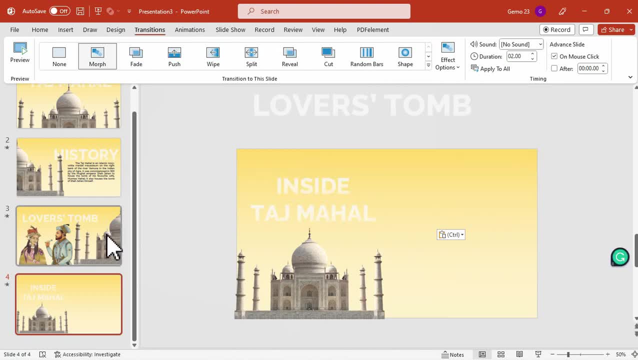 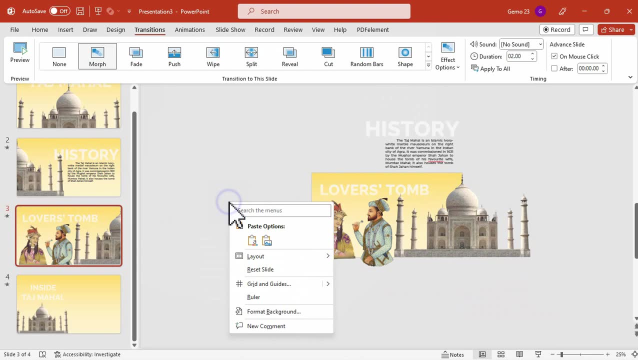 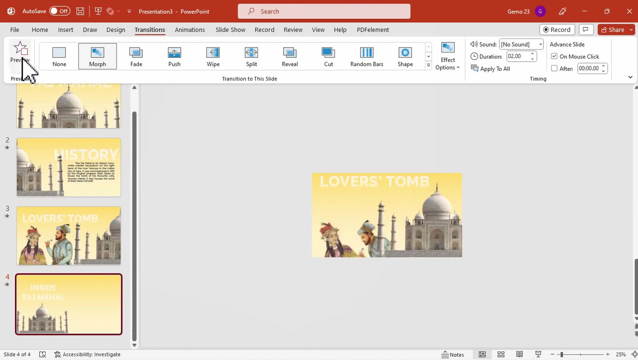 image and let's try to add this. Let's add this text: the inside Taj Mahal. So now let's copy that inside Taj Mahal text in the previous slide for the entrance morph effect. As you can see, the text came from the left side of. 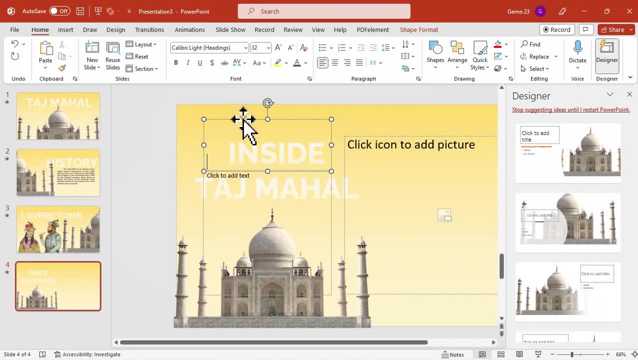 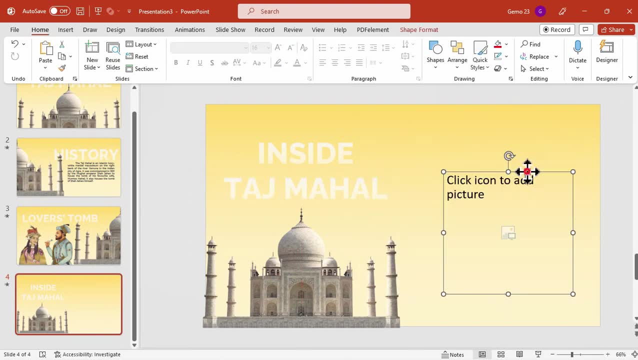 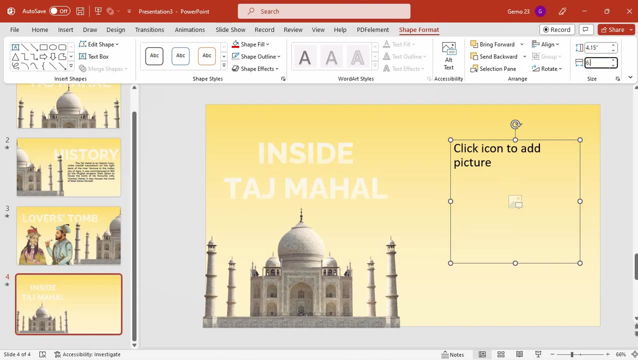 the slide. So we can also create a carousel effect with morph transition for images in Microsoft PowerPoint by following these steps: Insert the images you want to use in your PowerPoint presentation and arrange them in order you want them to appear in the carousel. So I will. 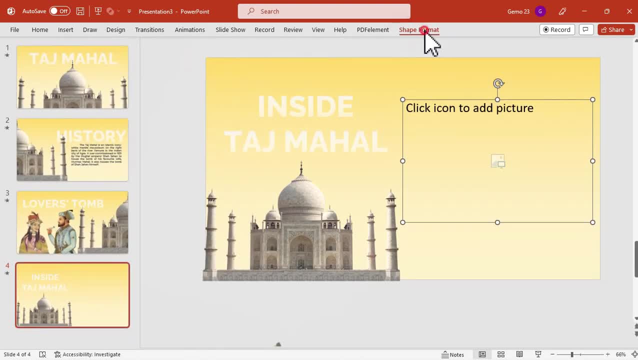 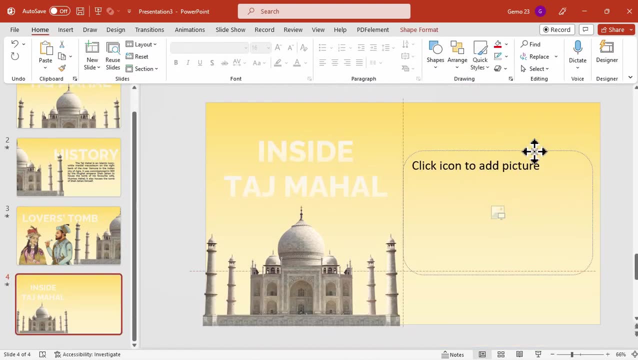 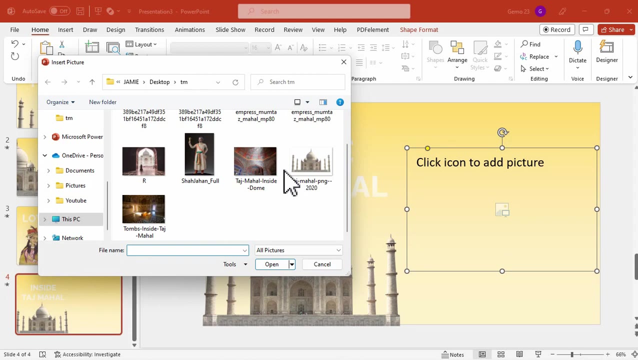 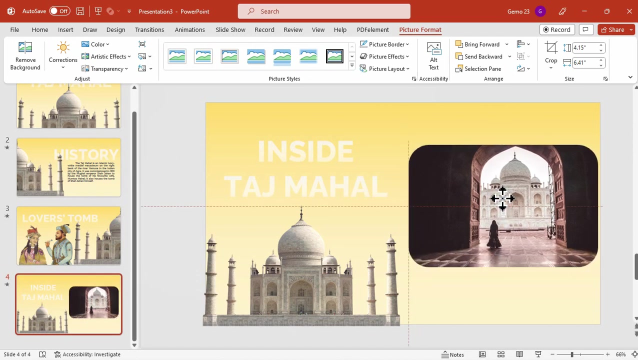 add this image placeholder and then change the shape into a rounded corners. So we will now add the picture inside the image placeholder. Let's select this picture and then we will add the picture of Taj Mahal inside. So here it is. Now you can place or adjust the position of this image. 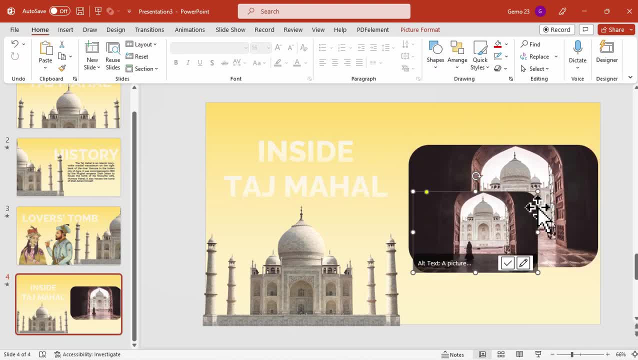 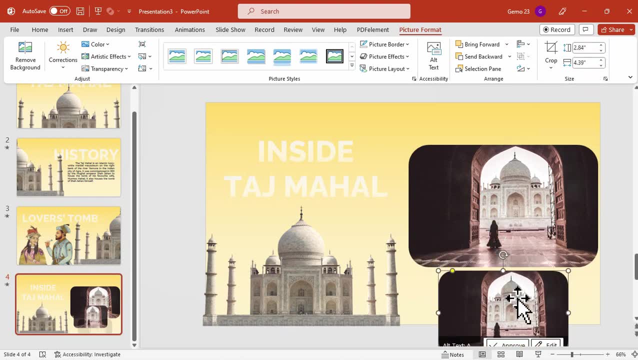 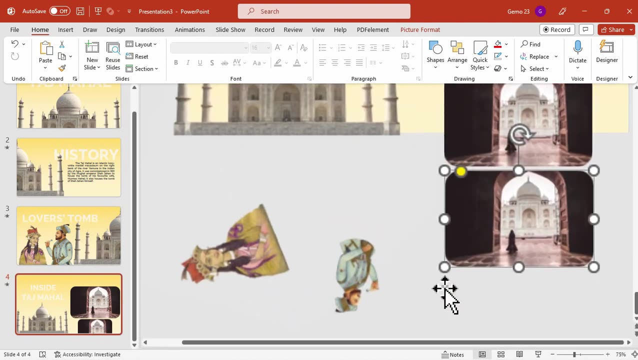 based on your likings, And let's try to copy that images and resize it, make it smaller. So we are doing this for the carousel effect And let's try to copy this once again and paste it. And now we will change this picture to a rounded corners. So we will add this image placeholder and then change. 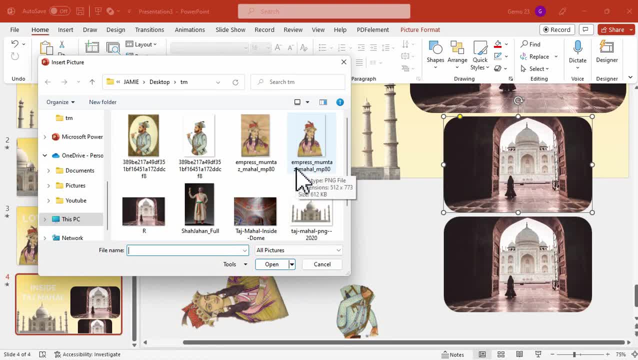 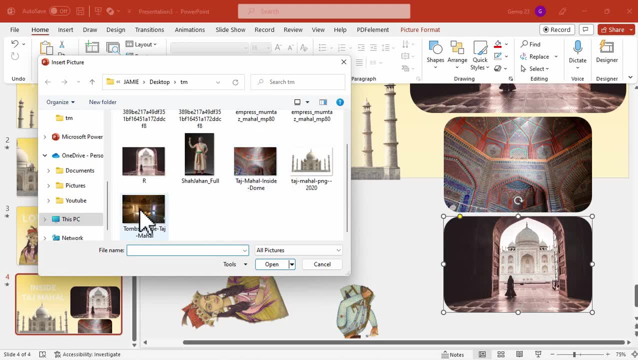 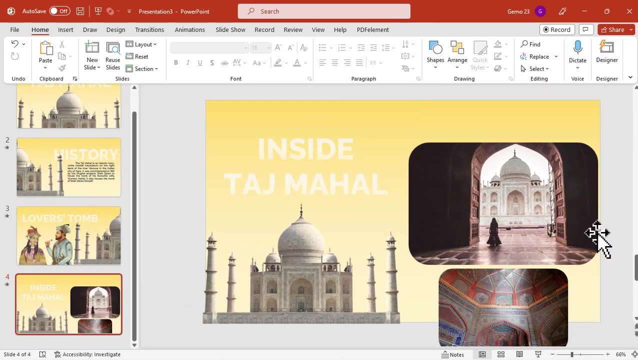 the shape to a rounded corners. So we will add this image placeholder. another pictures for our carousel: парuselfect, let's try this. another image for Taj Mahal inside. and four, the last image. So we have the pictures. Let me remove this. And now herea further picture said: That's more like what we are. 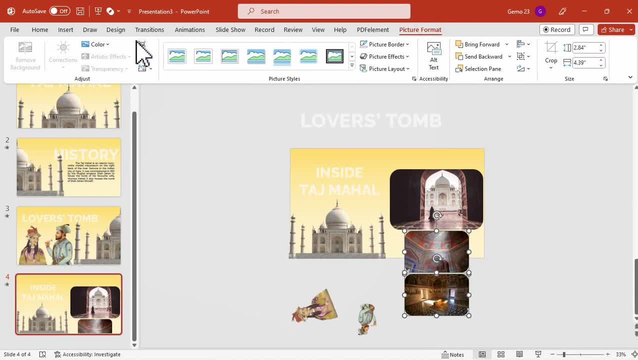 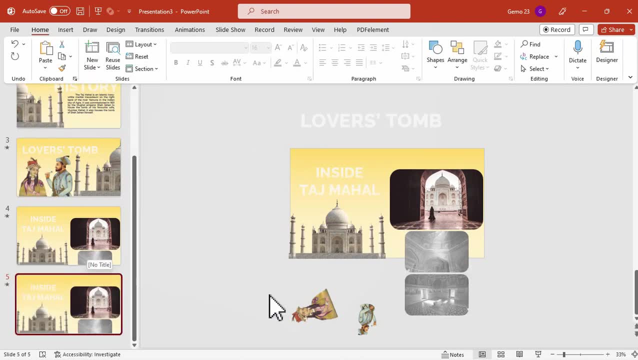 going to use for the carousel effect And for the smaller images, I will add this greying's effect. duplicate the slide and then you place the first image placeholder over the video picture without changing the crossiyet. OK, Then you are good to go. And what can we do now to remove all the pictures? 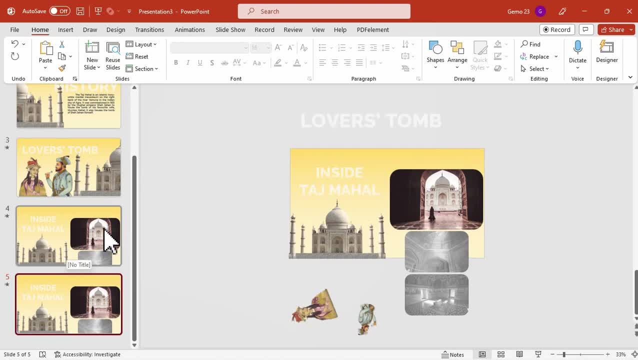 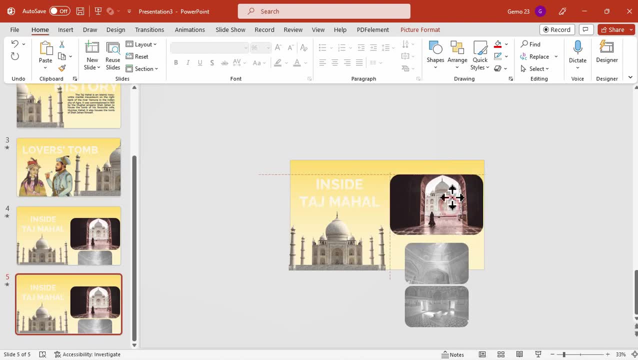 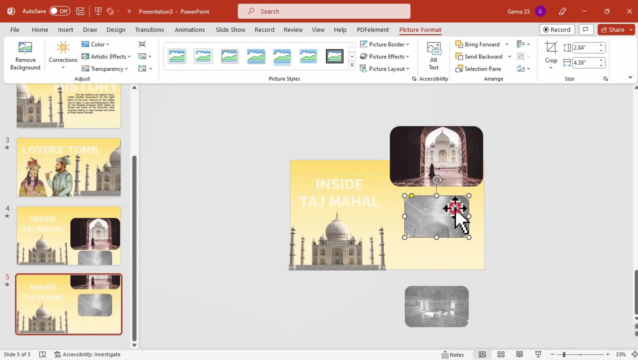 with the second image in the carousel. so we will just remove first these images and this text, since we don't need them anymore, and now we will adjust the placement of the image and the filter as well. so we will move the first image upwards and the second picture upwards as well, and then we will